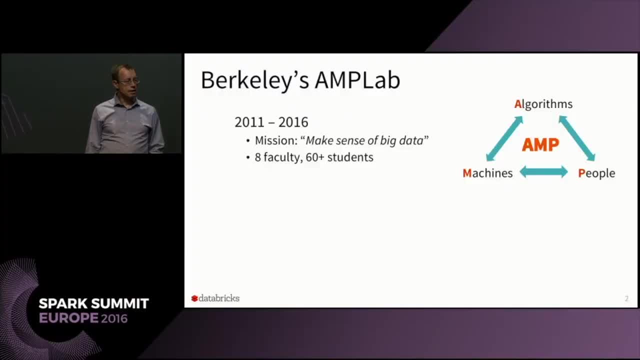 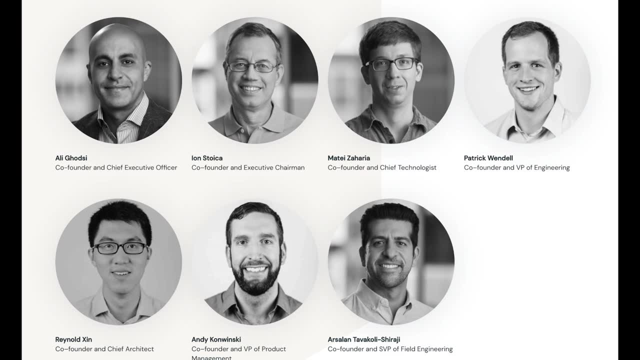 academia at AMP Labs in Berkeley University by several professors and TAs, Their names being Ali, Andy, Arsalan, Yon, Mate, Patrick and Reynolds, And I'm going to put their last names up as well. I'm going to butcher too many names And you can kind of get the sense as you scroll. 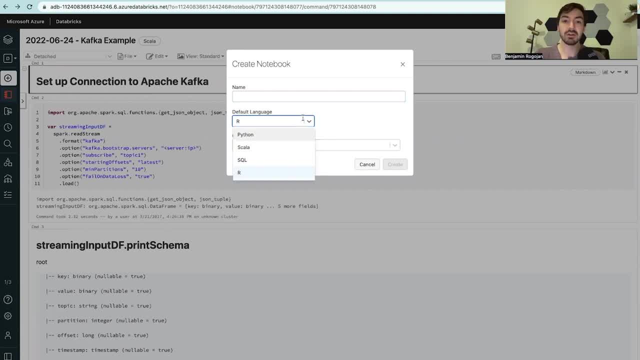 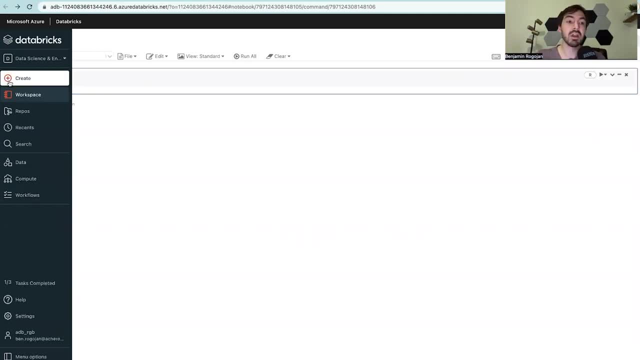 through Databricks product that it was really focused around the notebook. Yes, it was focused around Spark, but as you kind of go through it, everything is connected to the notebook. You create notebooks that then create jobs, that then create tables And everything was really developed. 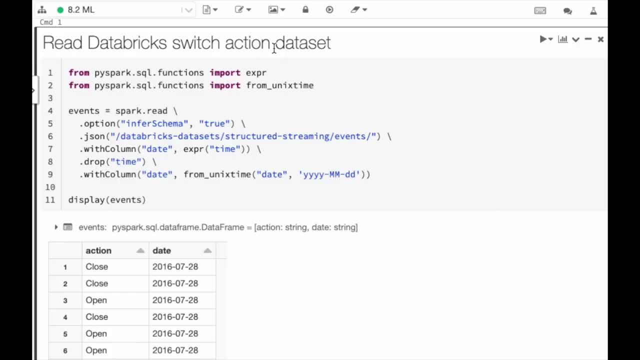 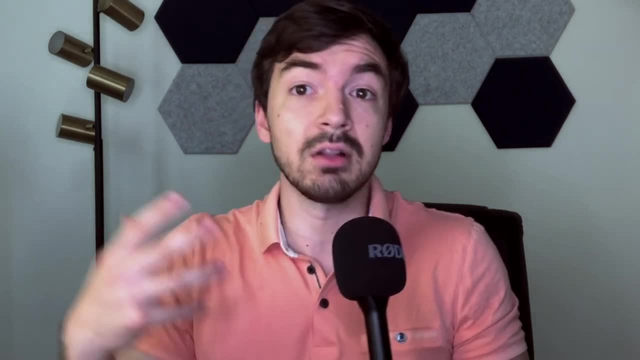 personally more for data scientists. It's again not meant to hinder anything or take a shot at it as a data engineer, It's just that's what it feels like. It's been further developed since then and I think it does a lot more now, But you can kind of feel like that's where it started, Like 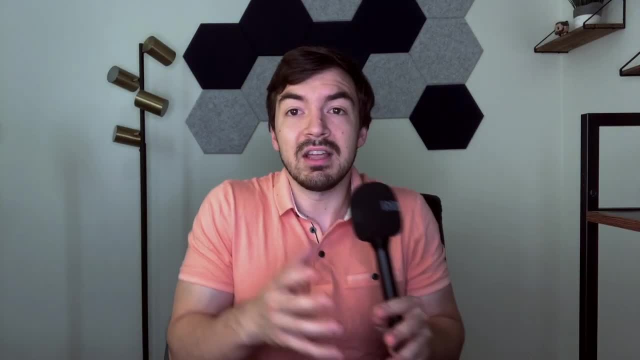 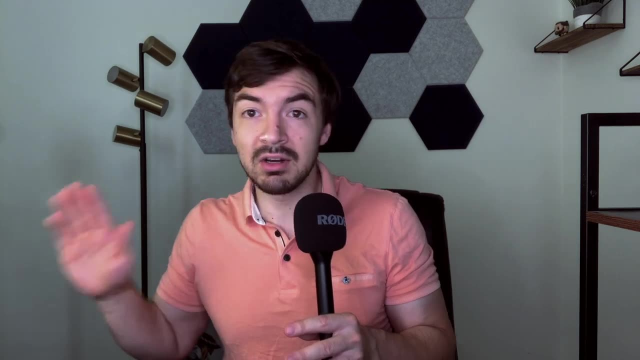 that was the center. That was its core, In the same way that Snowflake, when you look at it. its core wasn't necessarily these workbooks that it's now kind of going into. It was more around data warehousing, And that's why both of these solutions are now pushing. 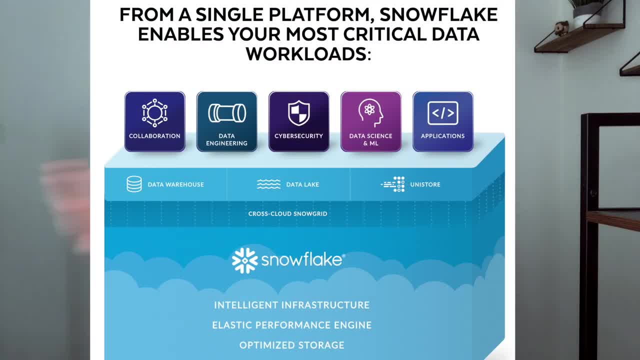 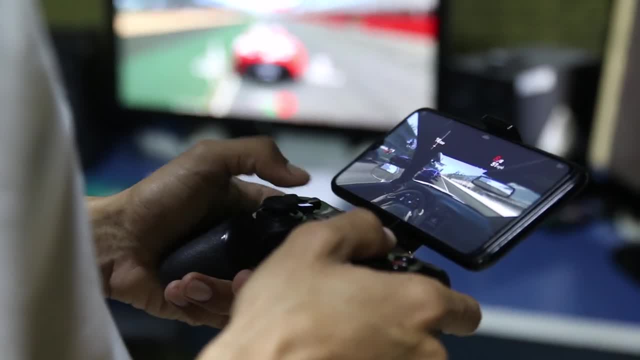 into becoming your data platform, your data OS, whatever you want to call it. That's where they want to go, because they know that is that next level. It's not just about their product and how you use it, but it's how you think about it. They want it to become. 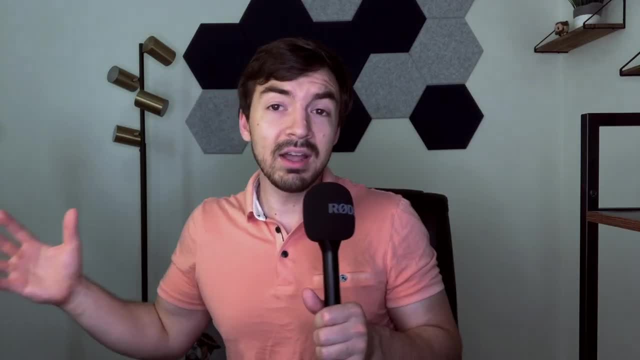 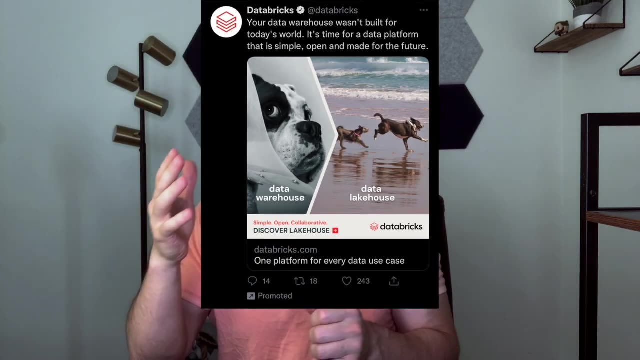 the thing that you go to to build everything else off of. That's why Snowflake has built Snowpark. That's why Databricks wants you to think of them as a data lake house, And we're going to talk about more of these differences, but it's important, I think, to understand that they're. 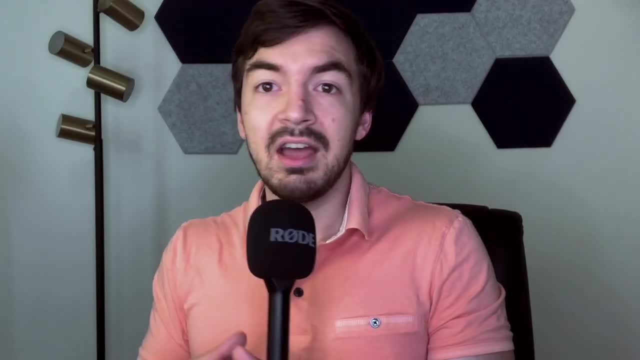 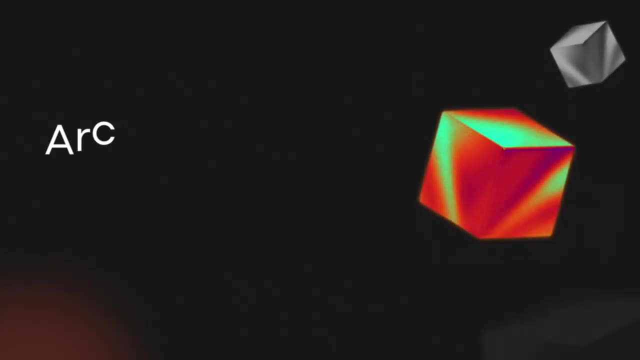 philosophically kind of different, at least from the start. They have a different approach to how they view data, And that's what I think is kind of pushing the rest of a lot of their differences. Now, with that, let's talk about infrastructure, The actual infrastructure and setup of these two. 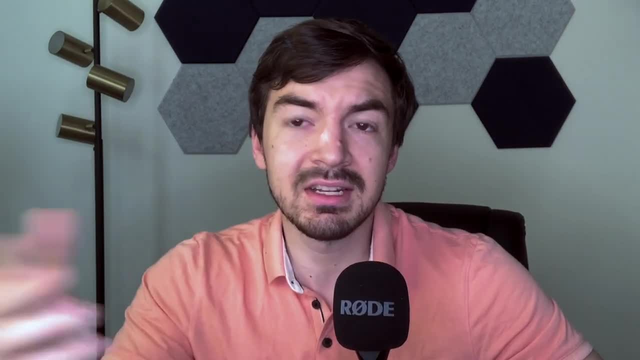 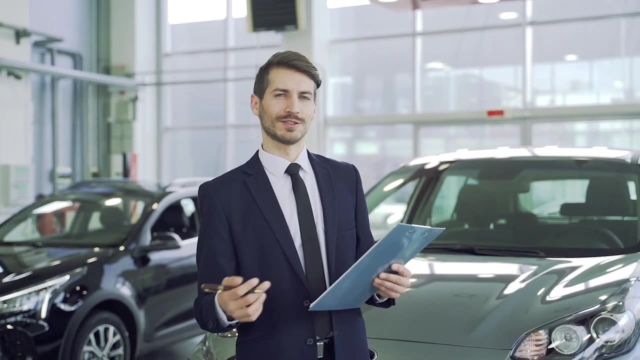 solutions is very different. Back in 2016,, I went to my first accidental Snowflake discussion, where they were basically just doing a sales pitch on Snowflake But honestly, early on it felt more like a discussion of solution, design or infrastructure. 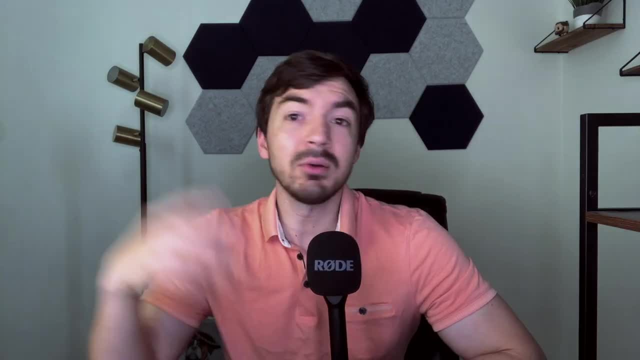 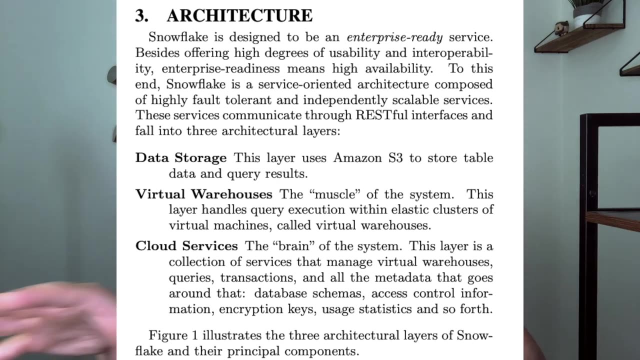 which was really fascinating, until they got to the point that it was clearly a sales pitch. They were talking about how they had these virtual data warehouses that would then basically sit on top of whatever kind of cloud storage you were using. I think at the time it was S3. I don't. 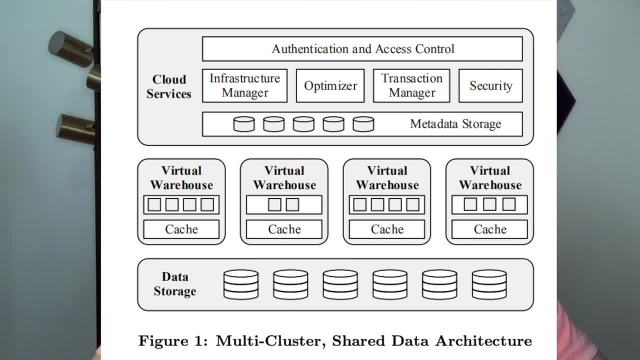 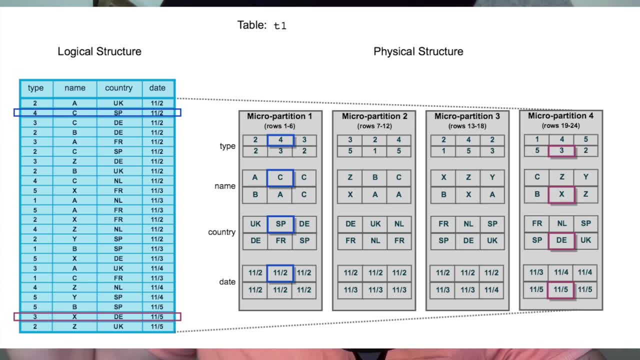 know if they had gone all the way to all of the solutions at this point. And then, on top of S3, they would sit and recreate micropartitions. Basically, these micropartitions would be how they would store your data and then they could index it And then they'd use these virtual. 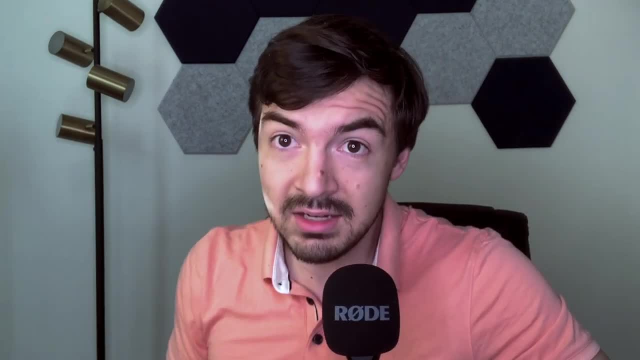 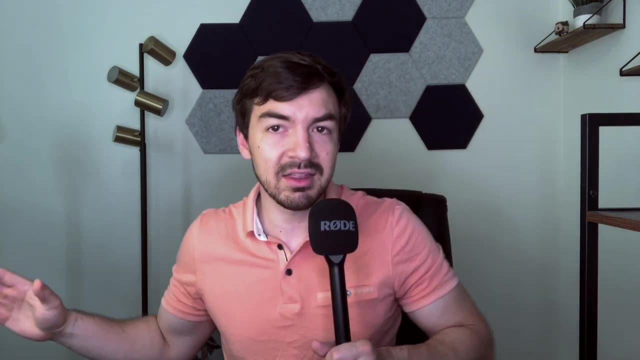 warehouses that they could scale up and down as needed so that you could have this auto scalability and use however much basically compute you needed. And that was the big thing. That was the big thing in. companies had been doing kind of some separation of storage and compute for a while. 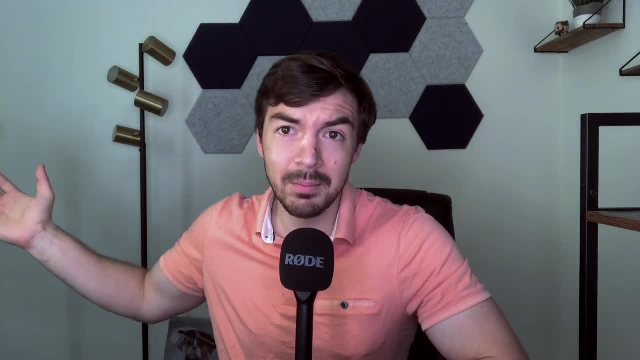 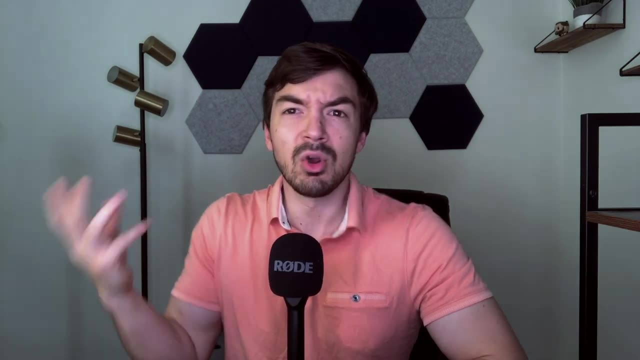 I think BigQuery was definitely first and there might have even been a company prior to this, But Snowflake was definitely the one that made it, I think, cool. They were the ones that made it the almost core of some of their products. It's a lot of what drove their product They had. 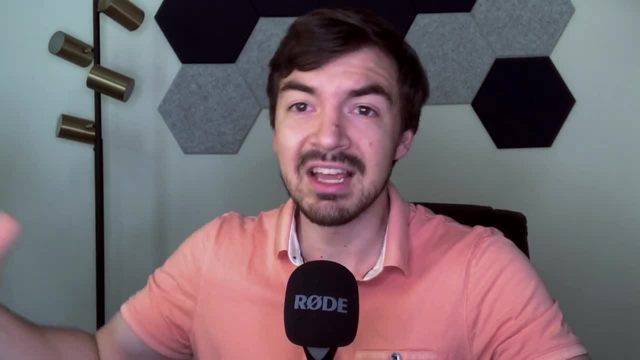 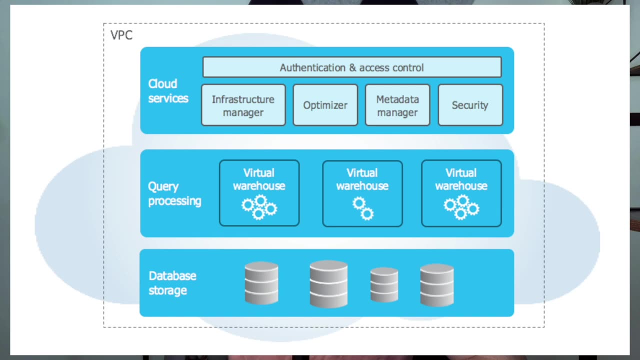 their micropartitions, which was a lot of how they had made sure they indexed and stored data in such a way that it was fast to pull up. But it was also that separation of storage and compute which you can kind of see in these diagrams that I'm putting up. 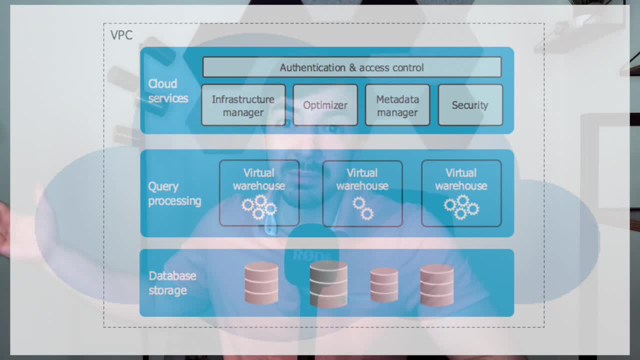 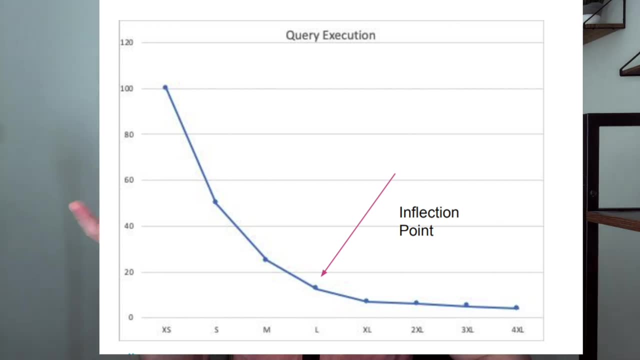 That allowed you to scale, Like, if you needed who knows how much compute- basically infinite compute- you could do it. You could do it tomorrow. You could just click a button, drop down to extra large and spend a ton of money and run whatever amounts of data you need. Now, when we go over, 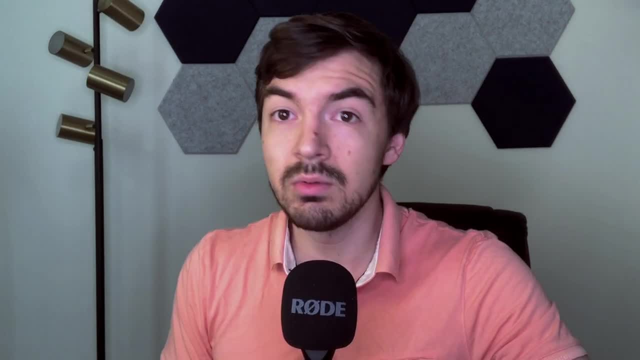 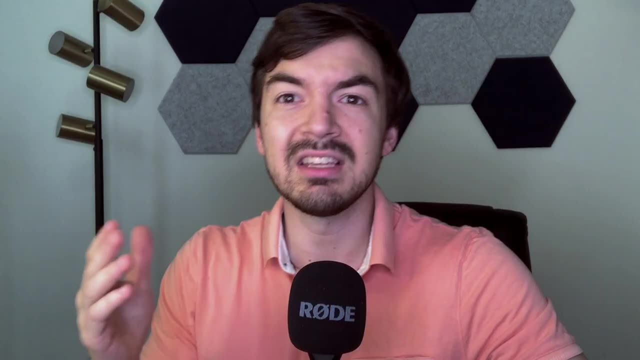 to Databricks. it's a slightly different approach. In Databricks, what you do is you create clusters that basically, are a representation of Spark compute. You can have them at different sizings. These will allow you to somewhat change sizes as you're running them, but you do need to create each of them. 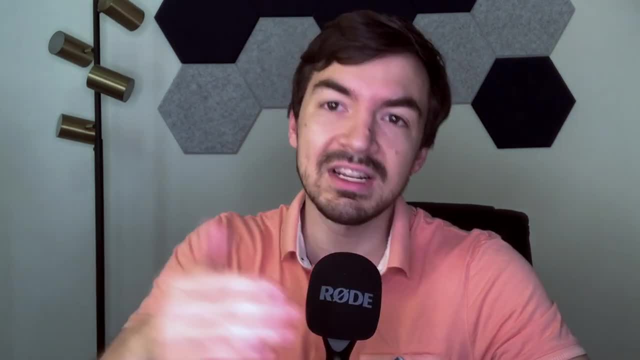 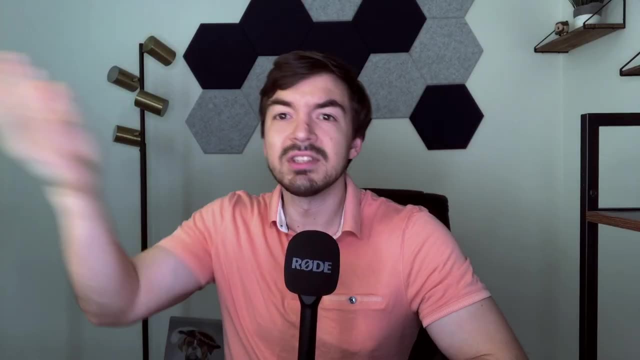 to create each one. it's somewhat similar to needing to create a actual warehouse in snowflake, but i feel like it just takes a little bit of an extra step because there's a little more in configuration. you'll see that when you're building out a spark cluster, but you'll see that their 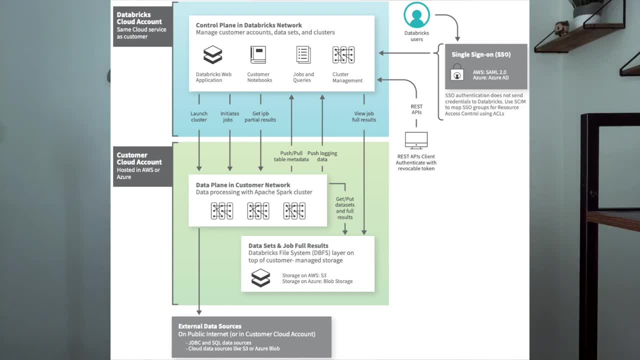 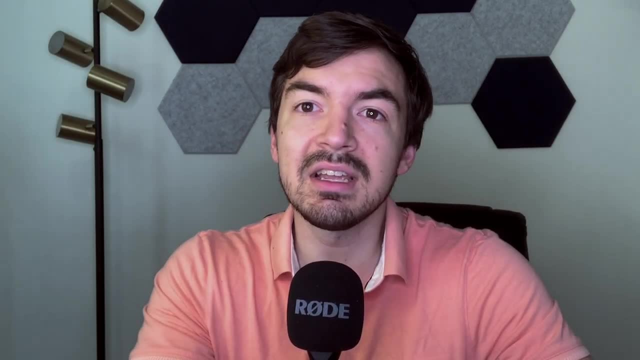 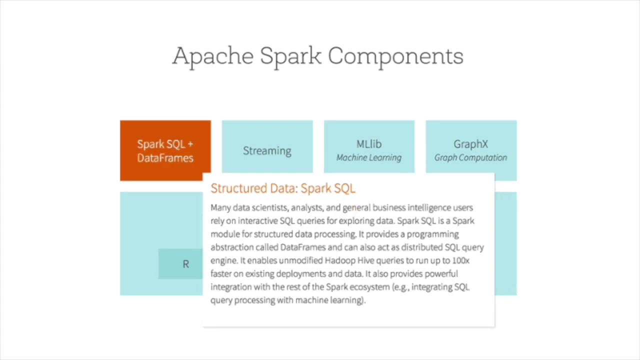 processing engine is spark, whereas snowflake had built a sql focus engine, databricks used spark and the great thing about spark, for anyone who's used it, is it is not language agnostic, but it is more of a polyglot kind of processing engine. meaning if you have scala, meaning if you have 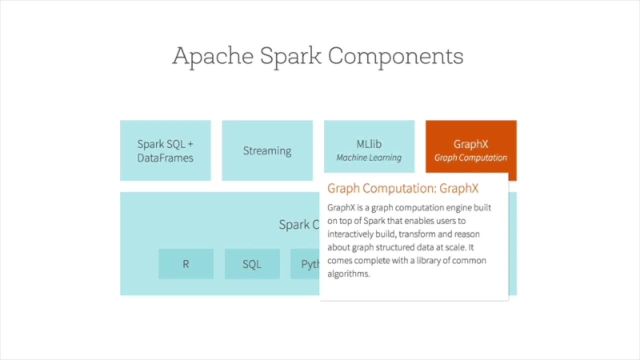 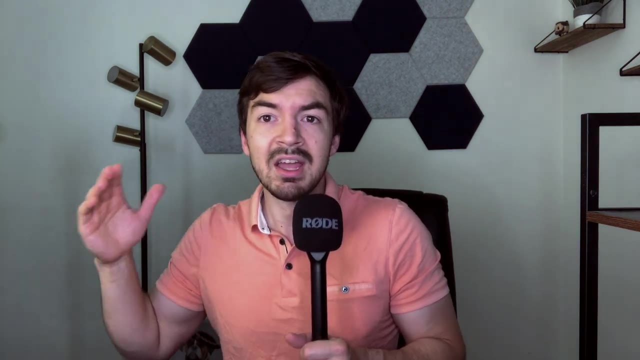 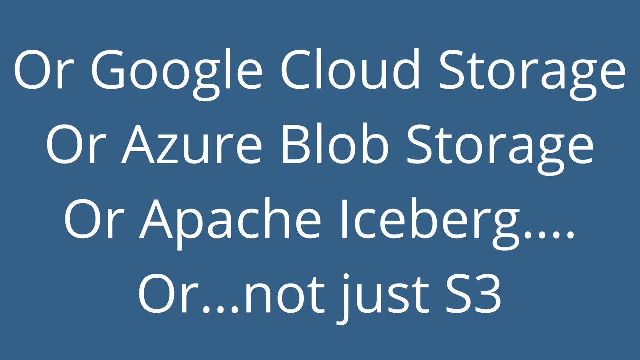 python, meaning if you have spark sql, all of that can be run through spark. that's great. it means you aren't limited to sql. it means you can run a whole host of other complex operations that aren't tied to sql. so, instead of doing what snowflake did, which was use s3, store your data, you're going to. 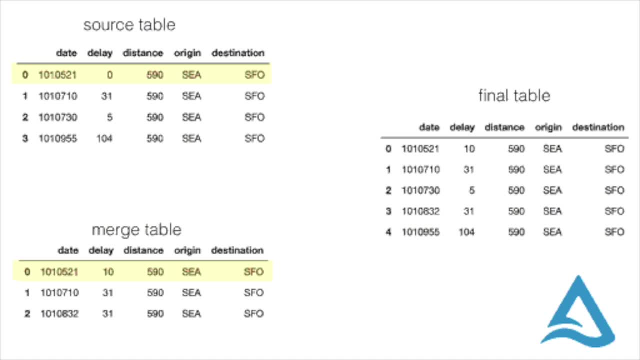 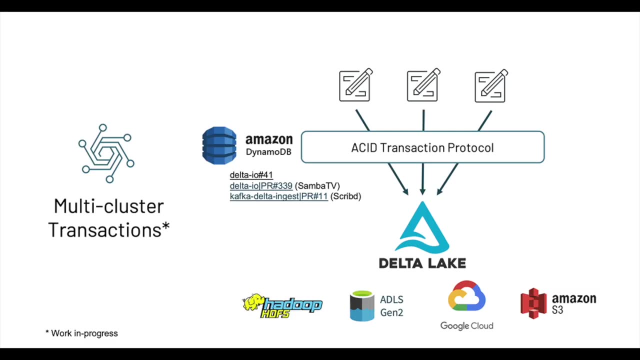 use delta link now. similar to snowflake, this infrastructure also separates storage and compute, so you can use spark. you're going to use delta link now. similar to snowflake, this infrastructure also separates storage and compute, so you can use spark to process your data and, in terms of storing it, you can use delta lake, which delta lake is databricks. 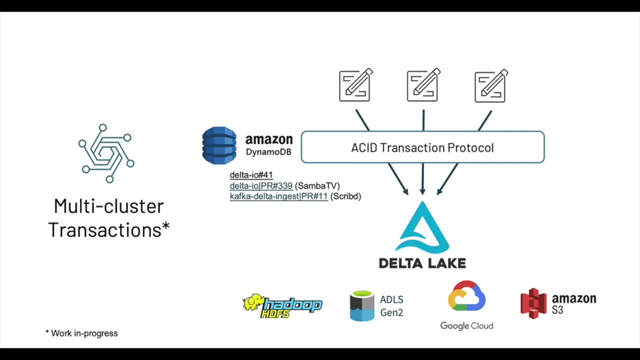 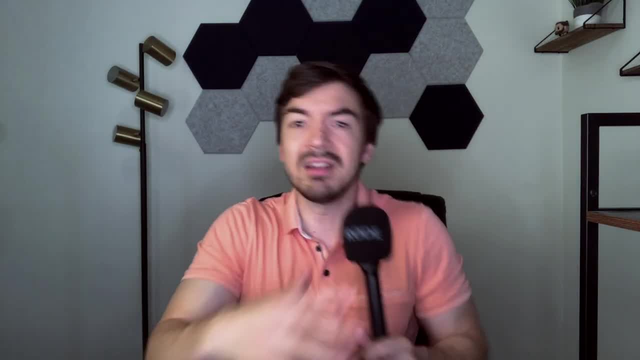 kind of storage solution. it provides you the ability to have acid transactions, which is great, so you can have the reliability of your standard database with a more data lake field- and we're going to get into that in a second, but that's kind of why databricks sells itself as a data. 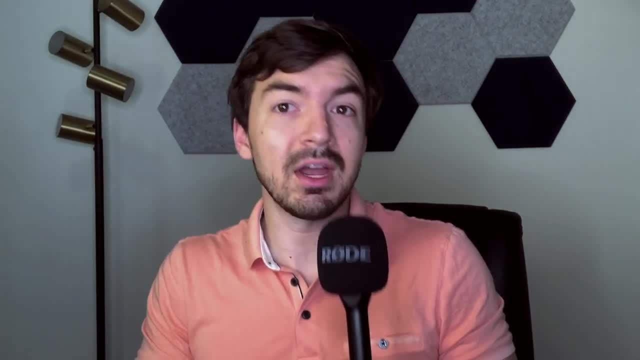 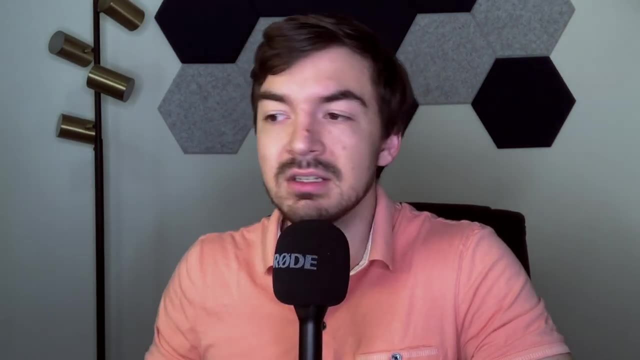 lake house and not just a data warehouse, because it does give you that ability to store data in varying formats. you can easily stream data into it. um, it's much more developed for that. you can do it with snowflake, and we'll get to that in a second. 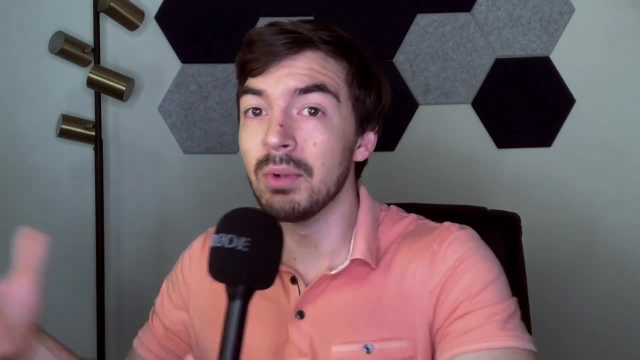 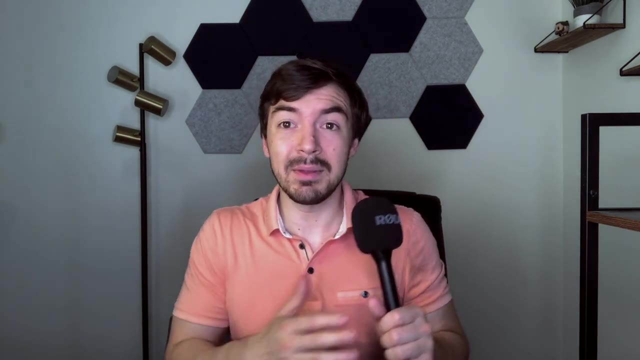 but definitely that's more of a native feature of databricks and kind of delta lake in itself, and it also lets you interact with data in multiple formats, such as parquet and abro, as well as storing data that's maybe semi-structured or doesn't have much of a schema defined early on. 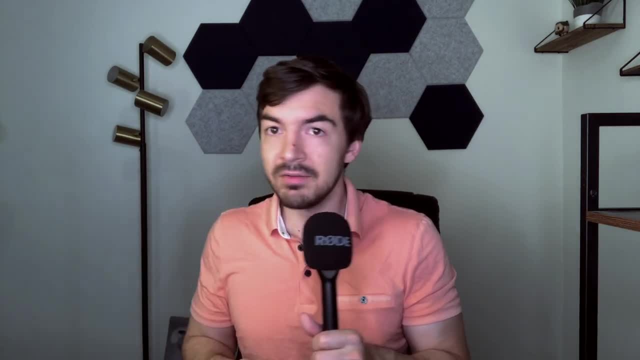 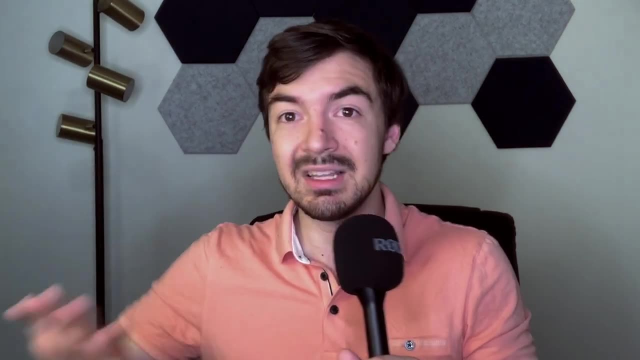 that you can then define later on as you're building tables off of your data, allowing you to unify kind of the data lake portion as well as your data warehouse portion, so you can kind of store some data, maybe more of an open format, and then push it into tables eventually. you recall from my prior video where i showed you that 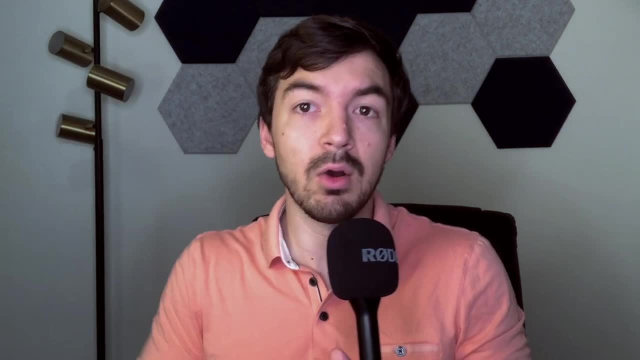 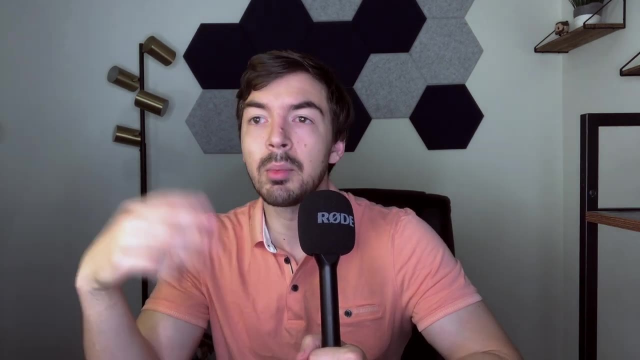 tables is something you can build, so you can start defining your tables over time rather than having to rush to them immediately. so if it wasn't clear, snowflake uses their virtual data warehouses and the proprietary sql engine to process your data that it stores, often in some 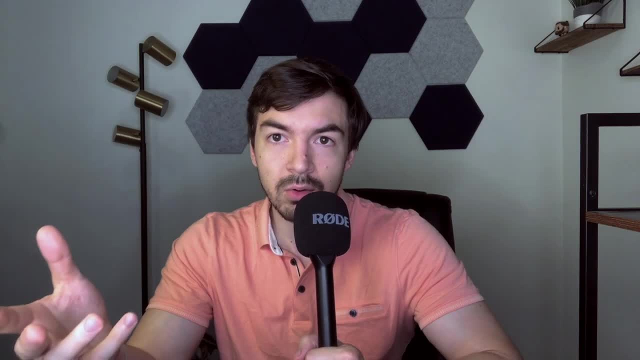 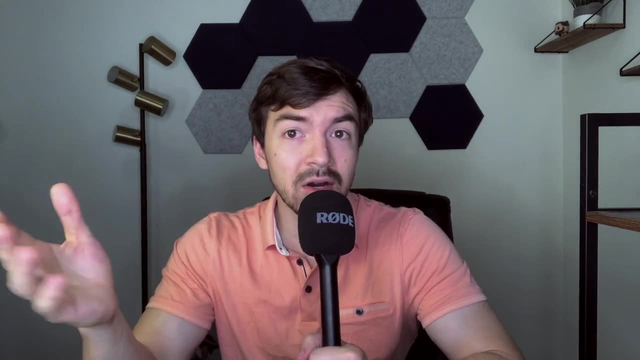 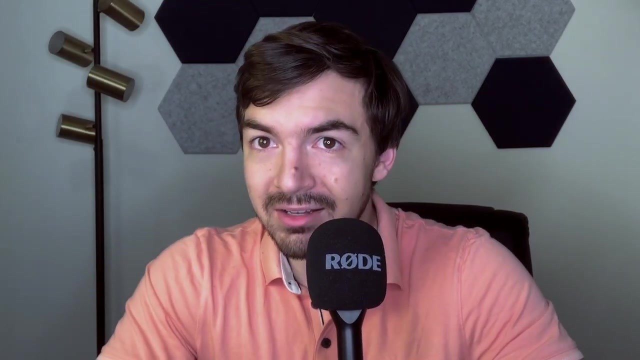 form of s3 or google cloud storage or azure blob storage in what they call micro partitions that they've indexed. so that's kind of how they've got it all set up, and databricks uses spark as a processing engine that sits on top of delta lake. from there, we need to talk about scaling, because 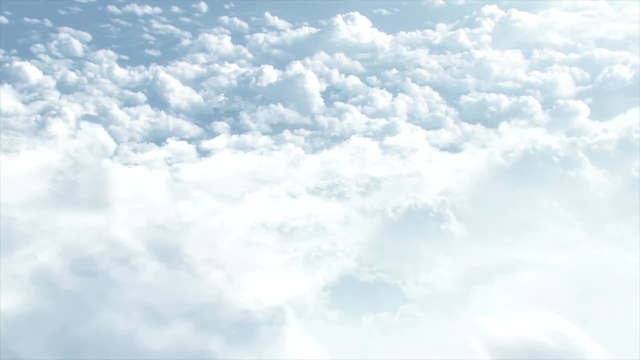 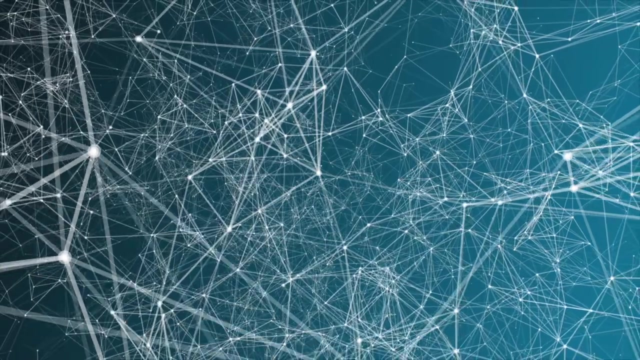 let's be clear. if you're building the cloud, one of the benefits that you would be amiss to not take advantage of is scaling as you need to now. with databricks you can scale pretty easily. one you can set it up to auto scale if you don't mind possibly accidentally running. 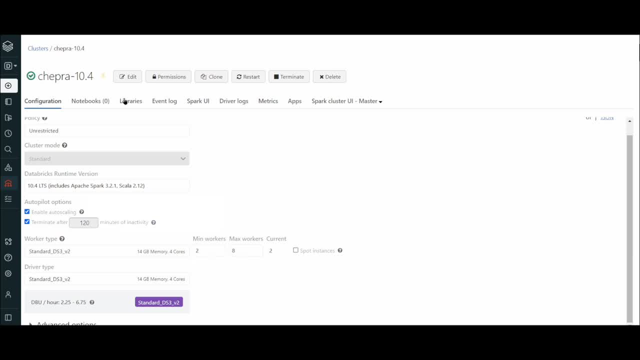 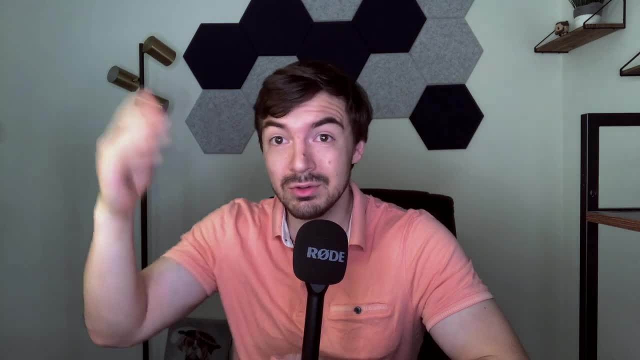 something at a higher cost. you can turn this off and on, but that is an option. you can auto scale so that it can process more data as needed, but in addition, you'd have to have some idea in terms of what all of these sizes mean. so if you scroll through, it is slightly more complicated. 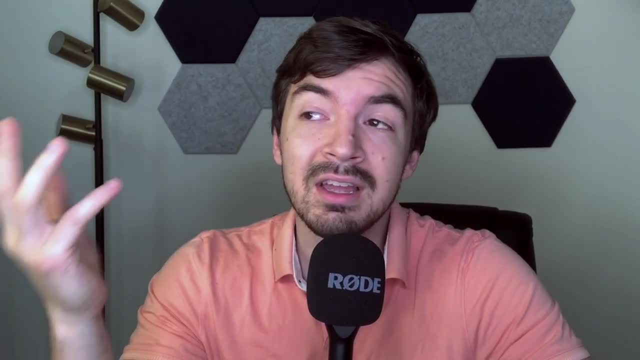 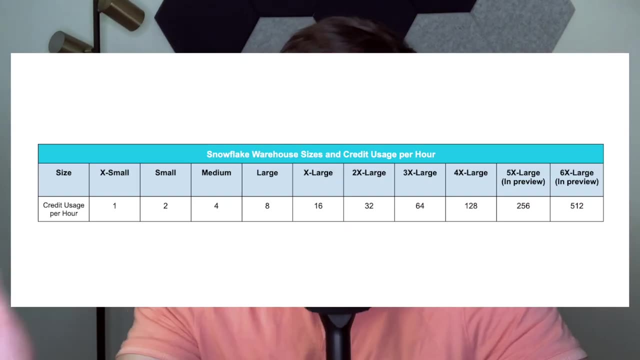 and it's not huge, but when we compare that to snowflake, they have done something that just simplifies it all together. they literally describe it as t-shirt sizes, and maybe that's overly simplistic for some people, but that's how they say. you know, it's extra small, small. 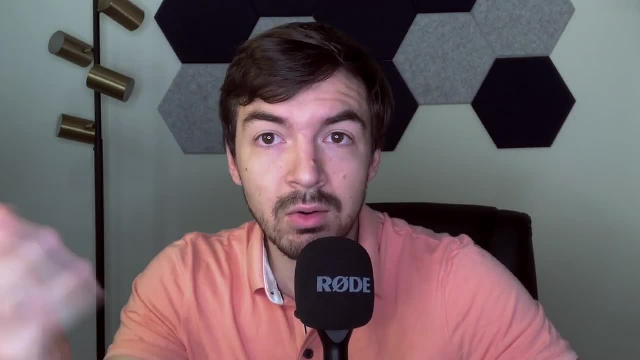 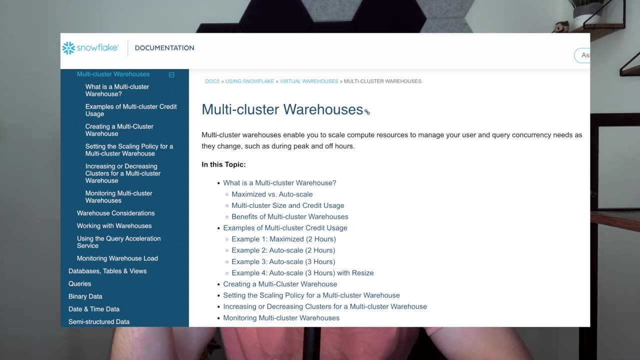 extra large. it's very easy to understand how to scale your snowflake compute and you can set it up to scale out to a multi-cluster warehouse to accommodate, you know, larger number of, maybe users or queries that are being run all at one time. so not only can you essentially take advantage of using more compute. you can start setting up multiple clusters of your warehouse to kind of run um more independently, so they're not bumping into each other, which is a common problem. if you've ever run anything on an on-prem data warehouse is that eventually you do hit a. 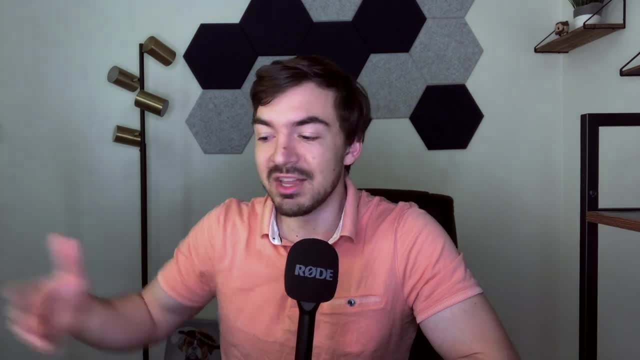 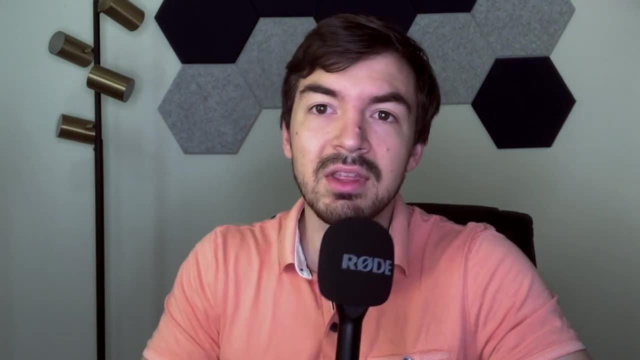 point where you know you can't just like copy another server, you can't just, you know, be like copy paste another server, but this essentially lets you do that can essentially let you isolate um compute and storage and so that they can kind of almost scale infinitely. there is a point of diminishing return for either databricks or snowflake. i'll 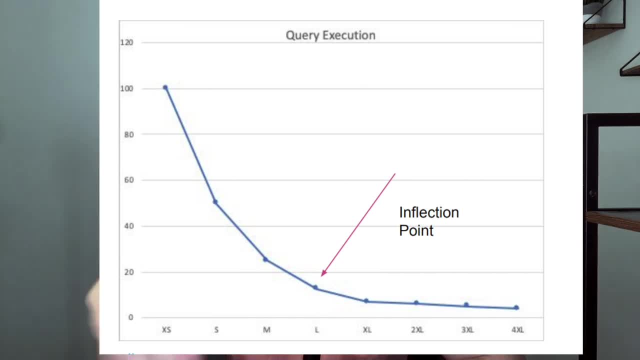 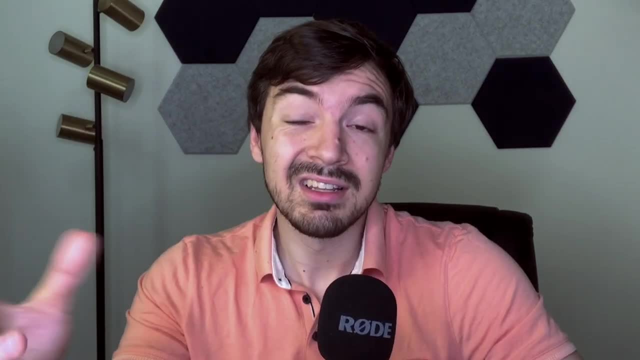 kind of put up a chart here. at a certain point you end up going from basically almost like doubling or quadrupling your speed to almost just having a minuscule amount of difference when queries get large enough. but that query can essentially run in isolation without blocking other people who might. also be running other analytical queries, so that's also another benefit. you might have a really long running query. that will cost you a ton of money, but it won't necessarily ruin other people's day. now i would love to talk about cost, but databricks and snowflake have done this. 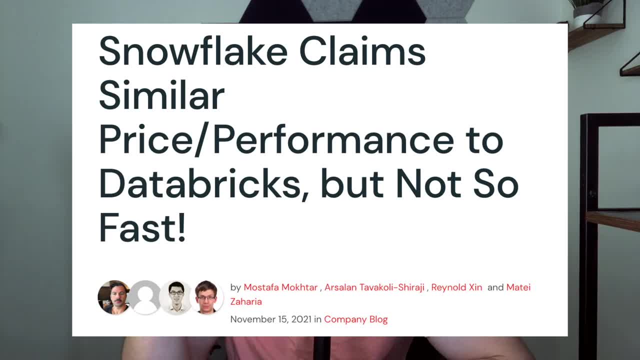 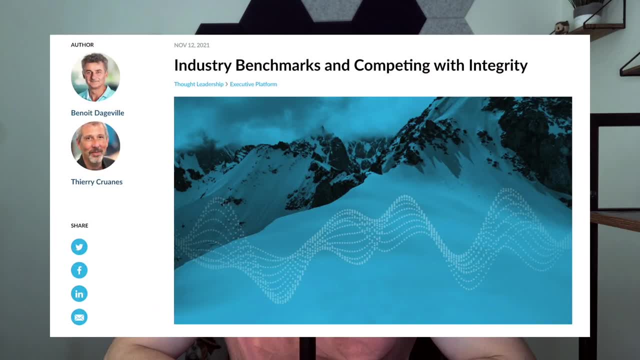 um, to death. i mean, if you missed it earlier- i think it was this year or last year, it was last year- the end of last year, snowflake and databricks decided to have it out with each other, as they both- passively, aggressively and maybe aggressively- wrote articles calling each. 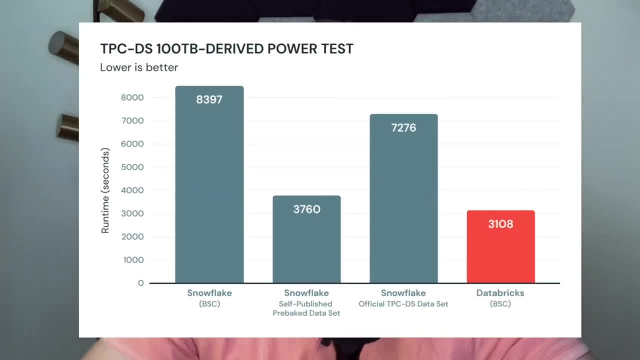 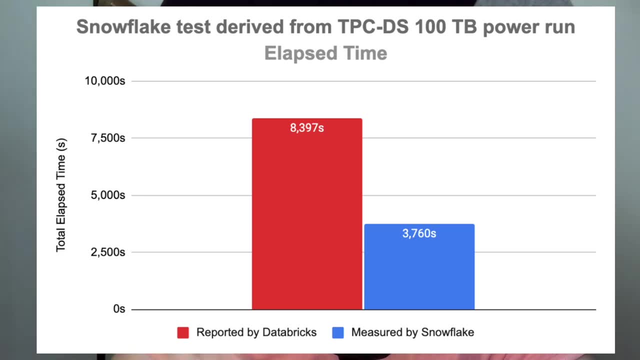 other out. they both essentially ran the tpc, benchmarking uh data sets, and both were basically pointing fingers and calling out. you know, bs, and there was a lot of fun that, if you missed it, i'm going to put up some of the articles and just the titles. one snowflake flat-out. 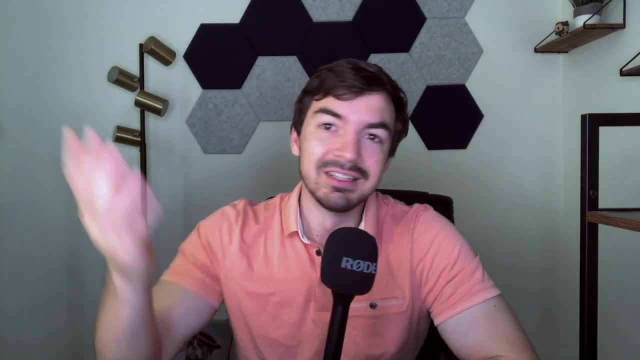 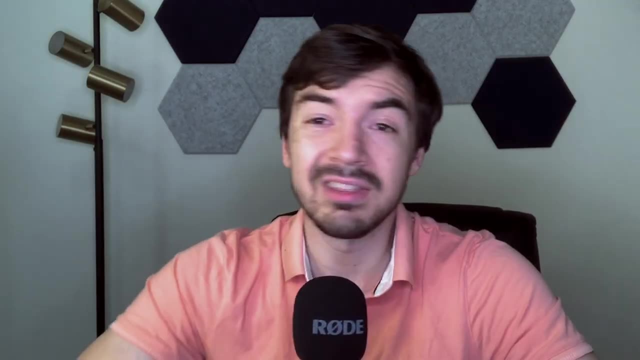 said that databricks was lacking integrity and databricks fired back saying that snowflake essentially lacked integrity and it was just. it was an interesting moment in time. but i do agree with one part that i read that snowflake kind of put out which was, if you read their article, that 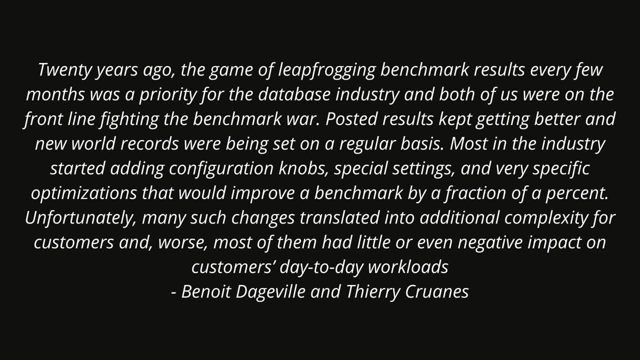 they put out that 20 years ago the game of leapfrogging benchmark results every few months was a priority for the database industry and both of us were on the front line fighting the benchmark war. skipping down a bit, they also added in. most in the industry started adding in configuration knobs. 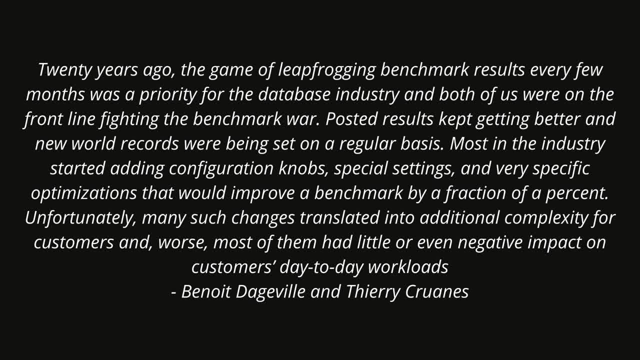 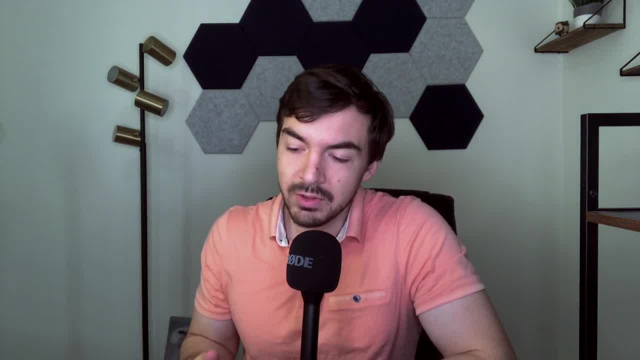 special settings and very specific optimizations that would improve a benchmark by a fraction of a percent. and this is kind of an extra point that i wanted to add in, which is especially with cost, when you add in all these like abilities to optimize and, you know, just configure things. 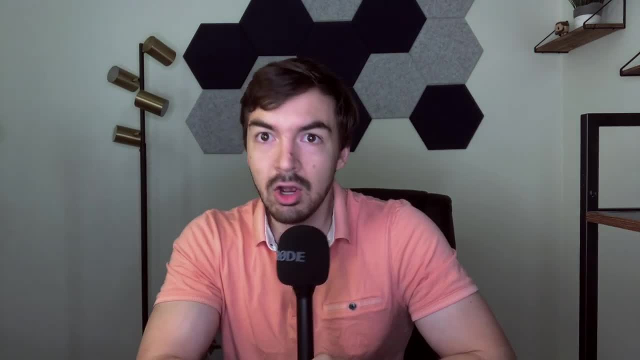 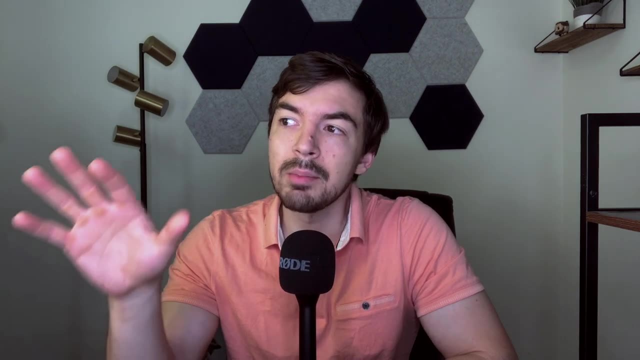 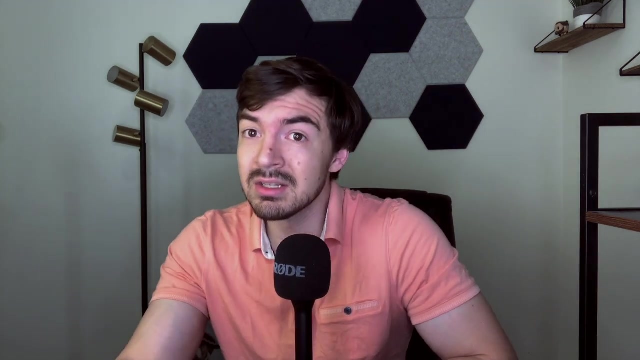 down to an even finer point. it often adds costs. in fact, this was something that's been known, i think, about oracle, where oracle was often really expensive to maintain, not just because of their licensing, but because it allowed you to fine-tune everything so well that you had to pay for very expensive consultants to manage it, and so there's a total. 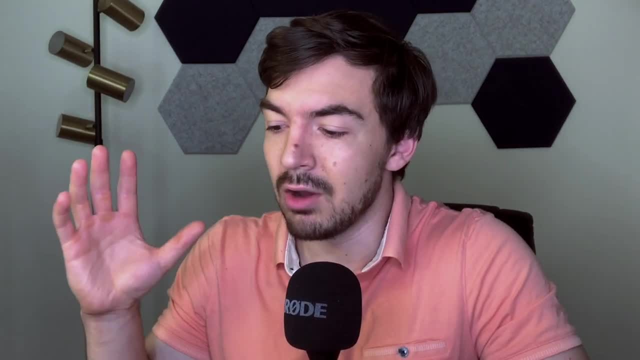 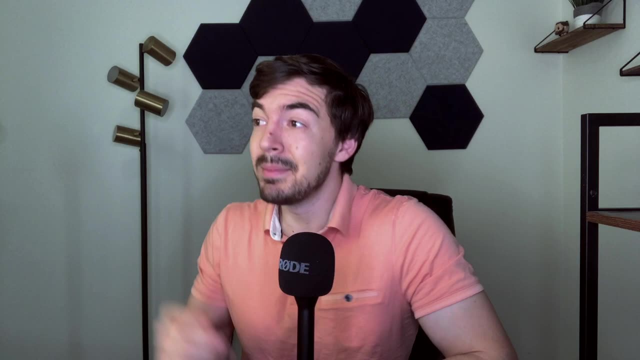 cost of ownership and total cost of basically managing and operating the systems that it's almost impossible to say personally which one's going to be cheaper for you, because at the end of the day, maybe you pay more for snowflake but maybe you have one less person that you have to hire. 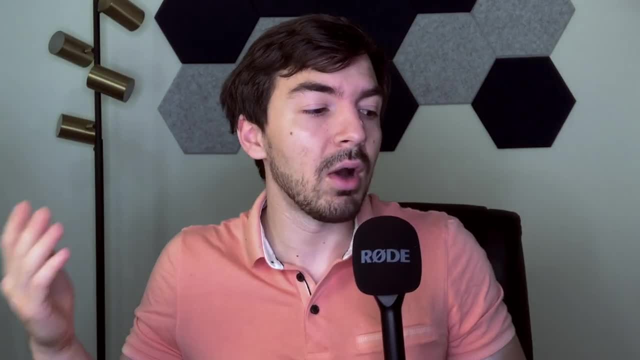 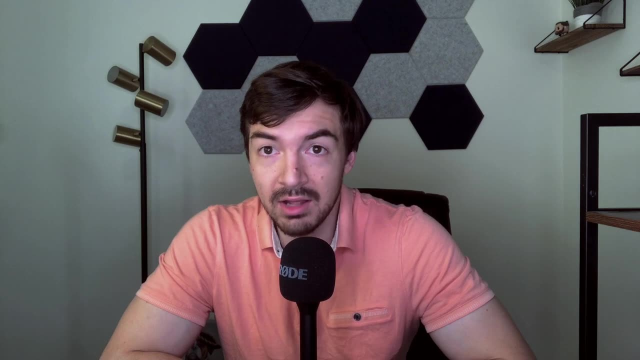 maybe i'm not saying that that's the case, but it could be the other way around too. so i'm not going to sit here and say that databricks is cheaper or snowflake is cheaper, because talent is a real cost and it's kind of hard to know how much talent you need. so we're not going to go too deep into. 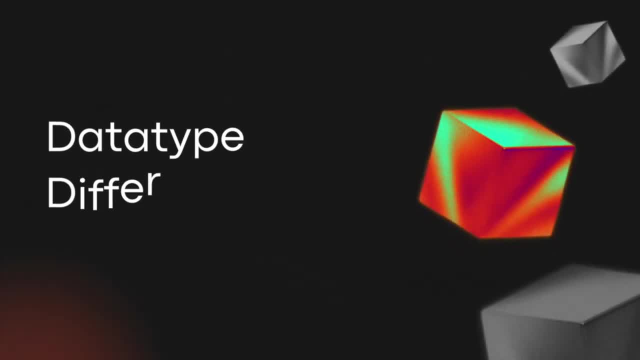 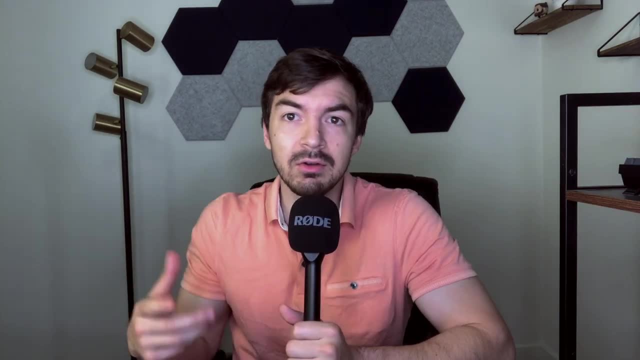 costs, but do read those articles. it's pretty funny. i'll link them below. now let's talk about data types. when it comes to snowflake, it does provide you the ability to work with several semi-structured data types, along with your kind of classic ints and floats and things of that nature, so you can. 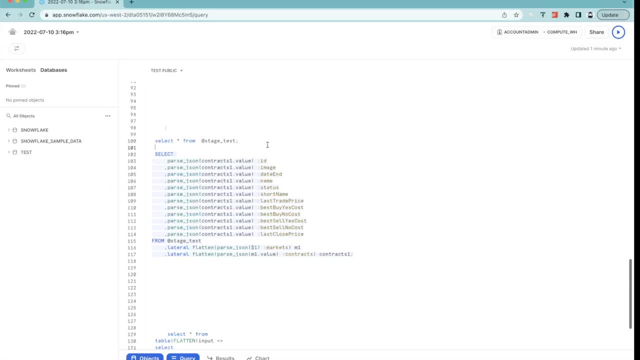 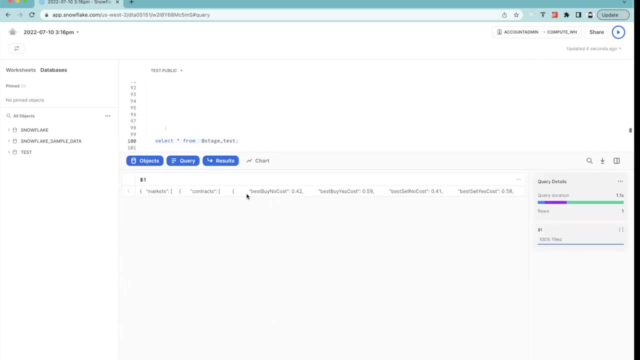 use the variant data type, object or array. in addition, on top of that, they actually allow you the ability to kind of work with json and even some xml through function, so you can actually store something like json in something such as the variant data type and then work with the json functions to actually call and interact with data that is in json format. now the 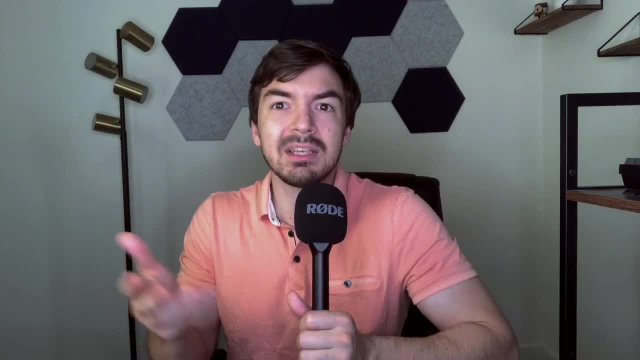 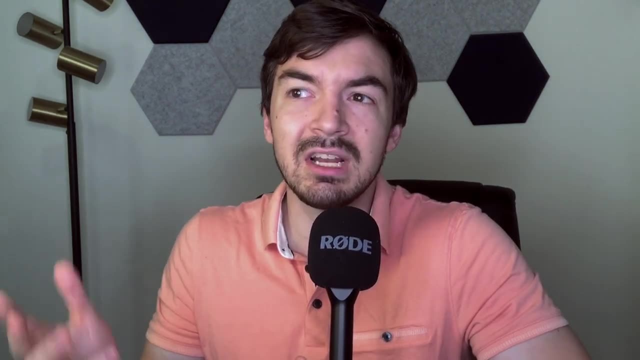 key thing here is it's actually, in terms of format, still semi-structured. completely unstructured data isn't necessarily that great in snowflake or even possible in comparison. databricks really isn't limited to data types. it's more like you can store your data in the format you need it and then 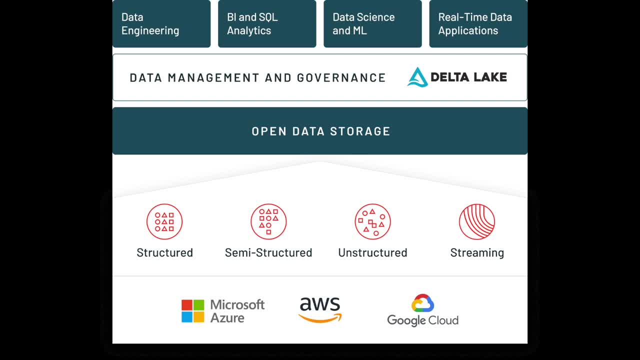 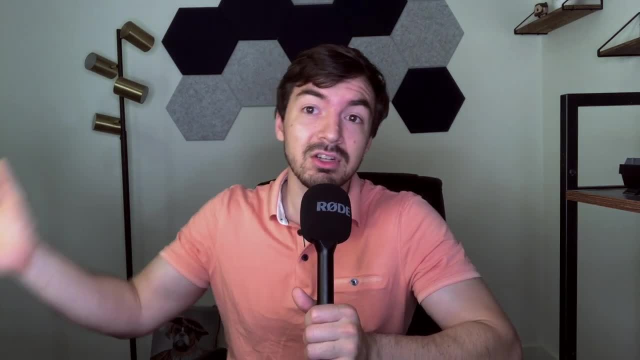 create tables from whatever that data is into some sort of schema really easily through databricks, and that's why it's kind of this data lake house, where it kind of gives you a little bit of both. you can have your data in one format and then eventually shift it over into something that is approachable by end. 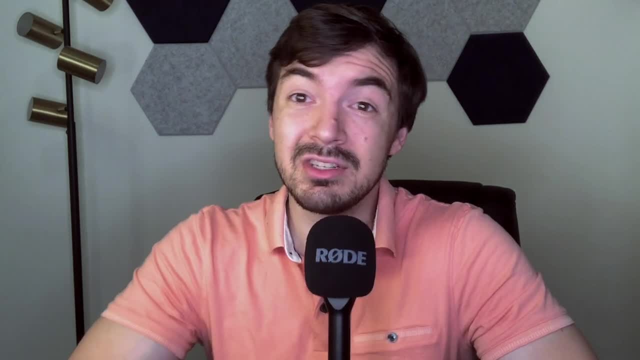 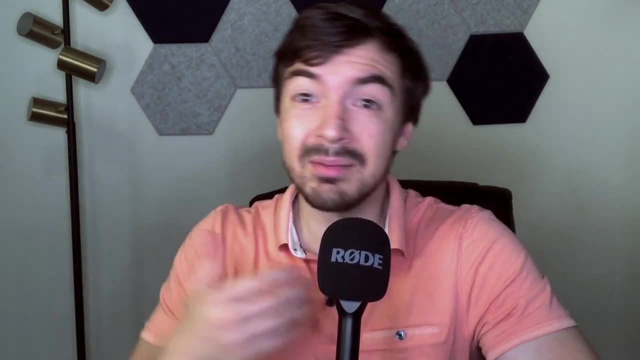 users, and that's what a lot of people do. that being said, i've seen a lot of people just use a hybrid setup, where maybe they store or process a lot of their more unstructured data in databricks and then store it in snowflake- and personally, that's, at a larger company, what i prefer doing. 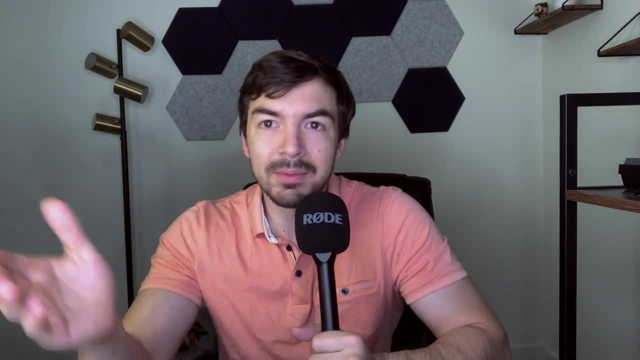 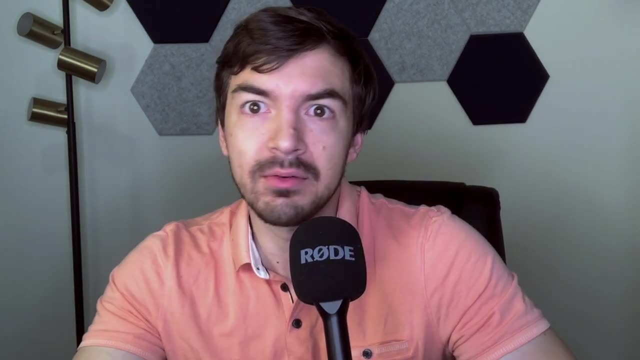 but that's just me now. i'm sure some of you want me to make a recommendation on which one of these is best. the easy answer is: it always depends um. i personally do like snowflake more for my classic connected warehousing. uh work um they are developing snow park which will let you run. 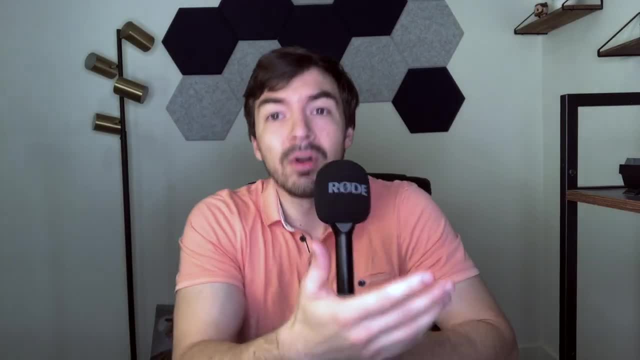 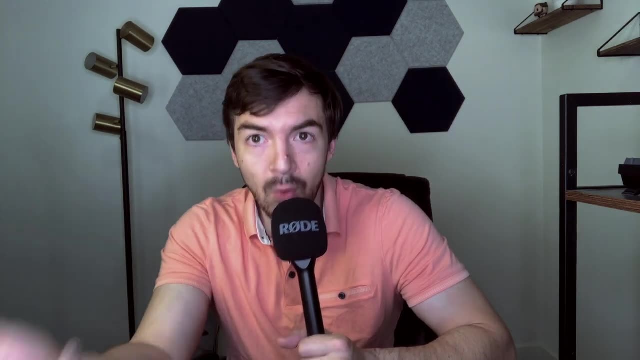 python on it, which will be exciting, and i'm curious to see where that goes, and i prefer more my ml workflows on databricks. i just think that's what it's built for and i like using tools for what they're for. obviously, both of these solutions want to kind of expand into each other's territory. 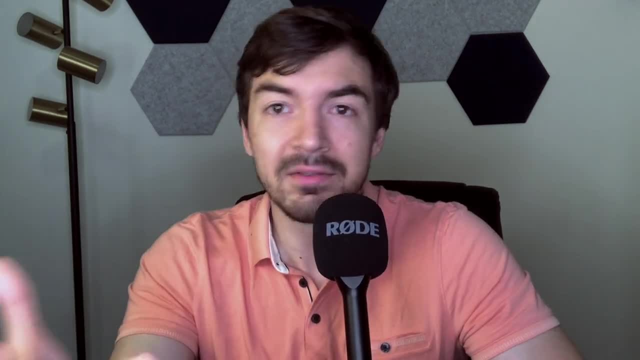 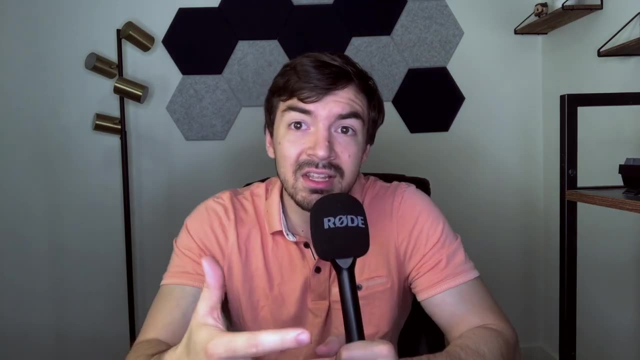 because that means more market share and it makes it probably easier for end users. but i think there will be people who prefer snowflake and always be people who prefer databricks. they're kind of designed differently. they're kind of focused around different concepts, even if they do. 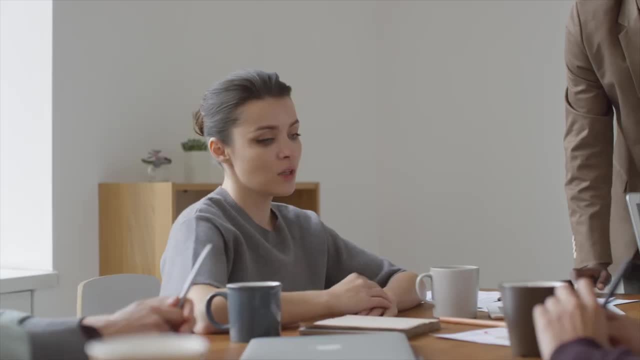 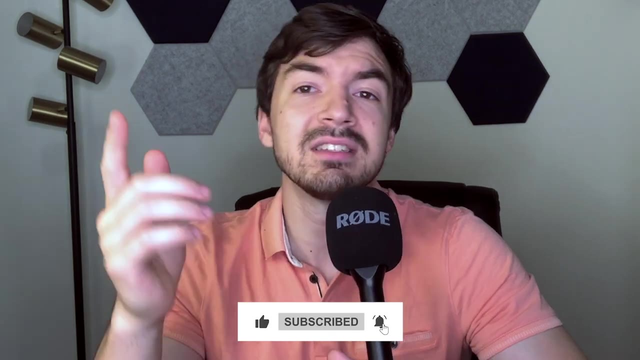 essentially the same thing in one regard or the other. finding the best one will really be up to you and your company's generalized use case, so i'll let you guys decide on what you prefer. with that, guys, thanks for watching and i will see you next time.